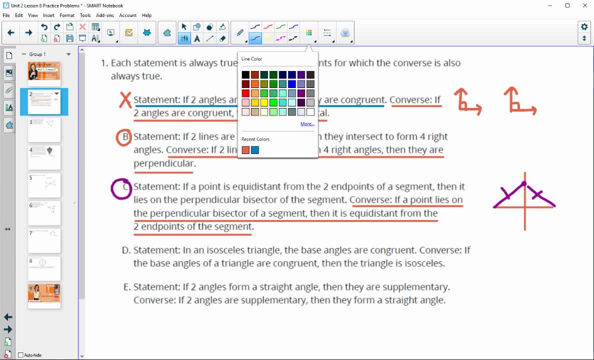 that is true D. the converse is, if the base angles of a triangle are congruent, then the triangle is isosceles. So if we have a triangle and we see that the angles are marked congruent, does that force it to be isosceles? 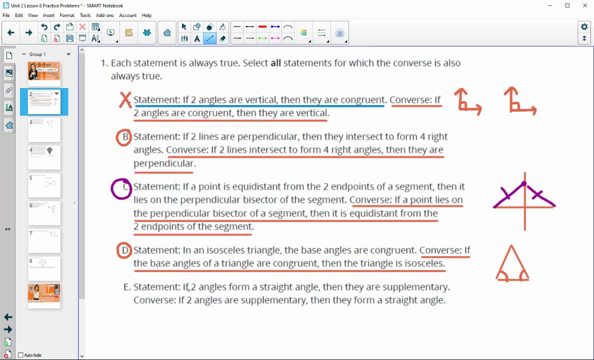 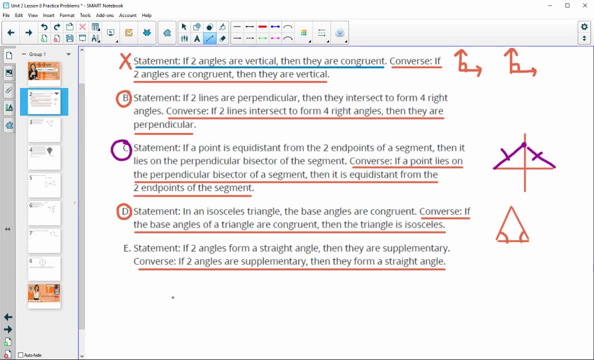 And it does So. that's true. E. if two angles are supplementary, then they form a straight line, form a straight angle. So the initial statement here was that if we have a straight angle, two angles that make a straight angle, then they're supplementary, which is true These. 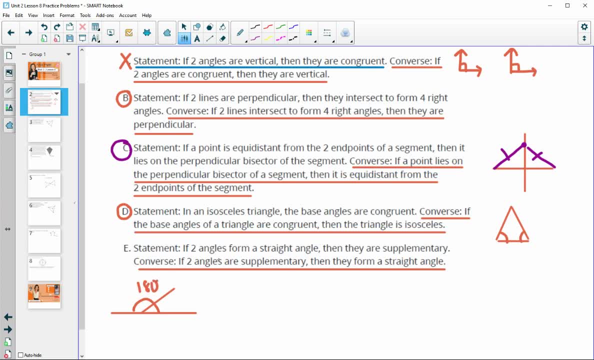 always total 180. But if we just know that the angles are supplementary, meaning that the angles add up to 180, do they have to make a straight angle? And that is false. So we could do this where I have a 120 degree angle and then I could have a 60 degree angle. These are definitely. 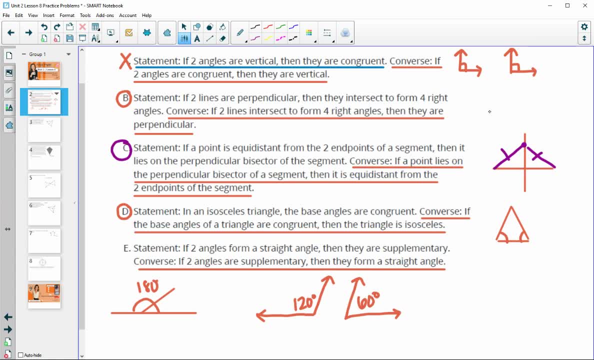 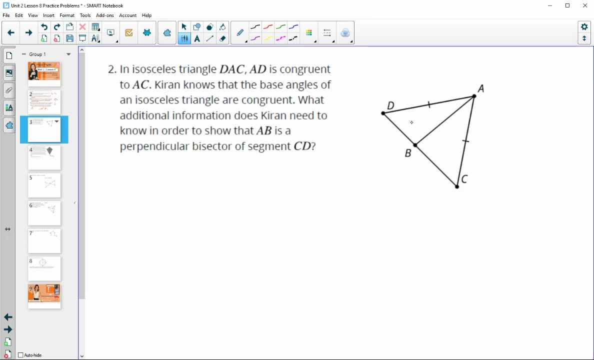 supplementary but they're not touching so they don't make a straight angle. This counterexample for converse A would also be a counterexample, so that's false. Number two in this isosceles triangle AD is congruent to AC. Kieran knows that the base 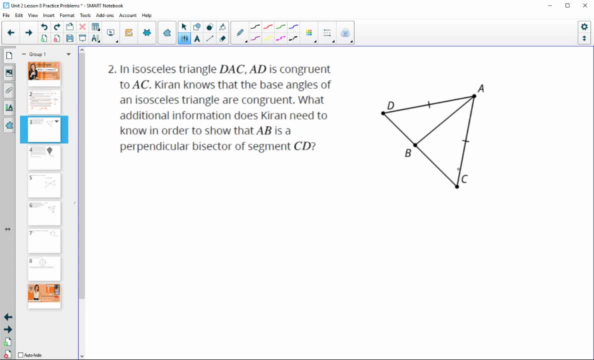 angles of an isosceles triangle are congruent. So across from these congruent sides are the congruent angles. What additional information does Kieran need in order to show that AB is the perpendicular bisector? Okay, so that this is the perpendicular bisector of this segment. So there's a couple. 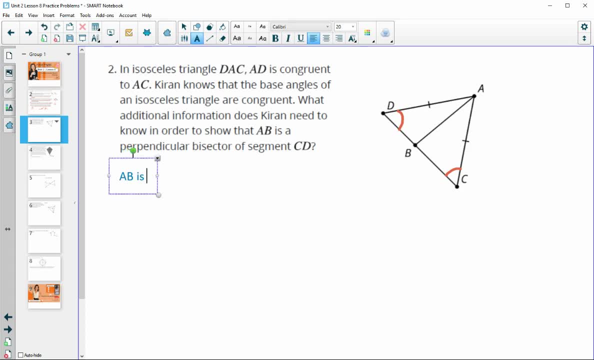 different things you could say here. So one would be that AB is the angle bisector of angle AC, And the reason that that would be helpful is if we had this angle marked congruent to this angle, then we'd have angle side angle to prove that the triangles are congruent, meaning that 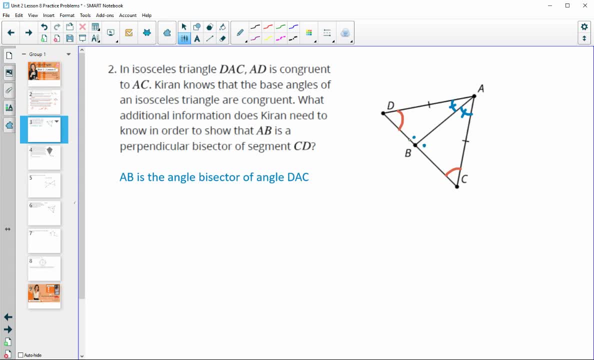 these two would have to be congruent to each other, making them 90. And then these segments would have to be congruent. so perpendicular bisector. So that's one thing we could know. We could also have that B is the midpoint of DC, And the reason that one would be helpful is that if we knew this was. 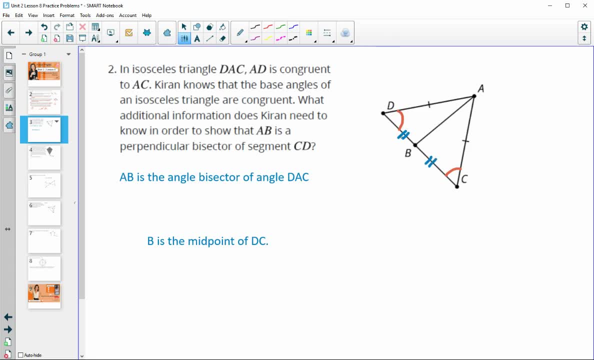 congruent to this, then we know the triangles were congruent by side angle side. So then you could get that those aren't equal angles that total 180. So those would be 90 as well. So this one would allow us to use angle side angle. This one would allow us to use side angle side. 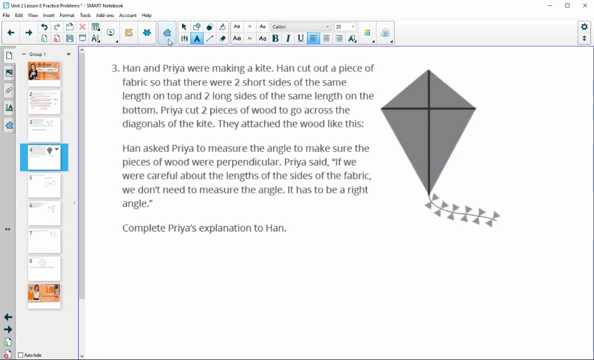 All right. number three: Han and Priya were making a kite. Han cut out a piece of fabric so that there were two short sides of the same length on the top. So he cut these two to be the same length And to long sides on the bottom to be the same length. 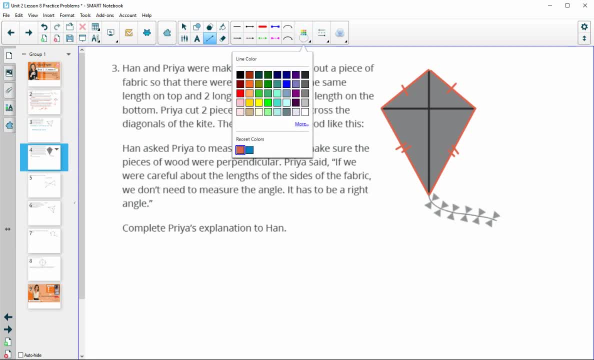 Priya then cut pieces of wood to go through, to go across the diagonals of the kite, so here and here, And then they attach the wood like this. So Han asked Priya to measure that angle, to make sure the pieces of wood were perpendicular. so asking her to measure, 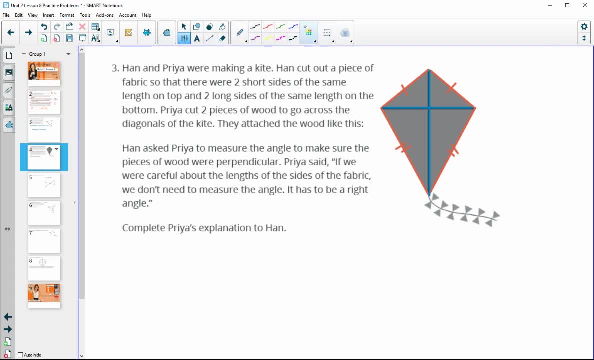 the angle to make sure the pieces of wood were perpendicular. So asking her to measure at this angle, this angle to make sure that everything is perpendicular. So asking her to measure, So asking her to measure, her to measure to make sure that this is a 90-degree angle. Priya said, if we were careful, 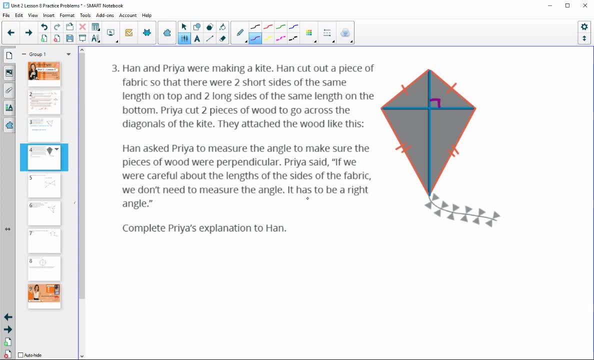 about the lengths of the sides of fabric. we don't really need to measure. It has to be a right angle. So complete Priya's explanation to Han. So why is that true? And so I'm going to put some letters on here so that we can more easily describe this. So if I look at this and I put 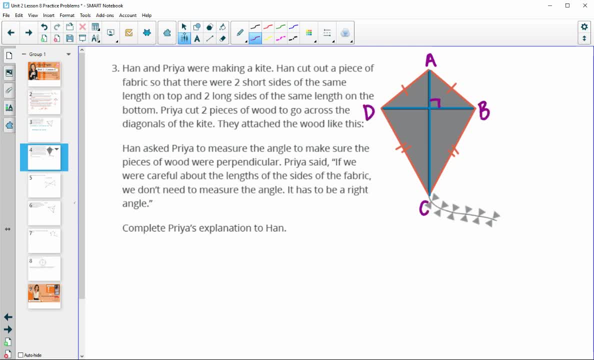 A, B, C, D here. Okay, then we'll go ahead and type out this explanation. So since A and C are the same distance or equidistant away from B and D, they must lie on the perpendicular bisector of segment. 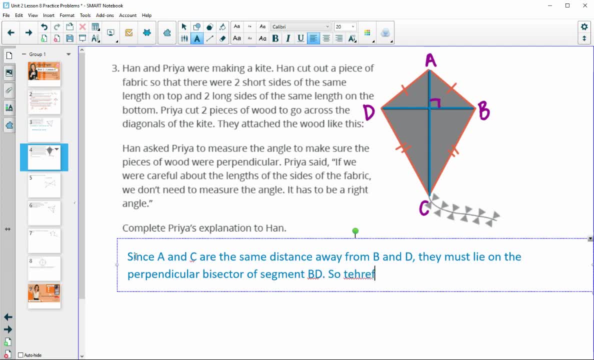 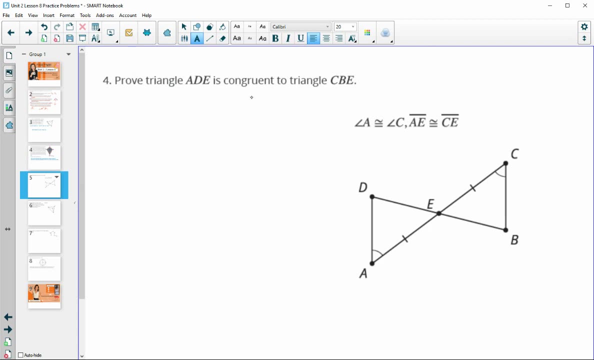 B, D, And so therefore A, C must be perpendicular to B D. Number four prove that triangle A, D, E is congruent to C, B, E. So they give us some information here. So let's start our proof with that. So we know that angle A is congruent to. 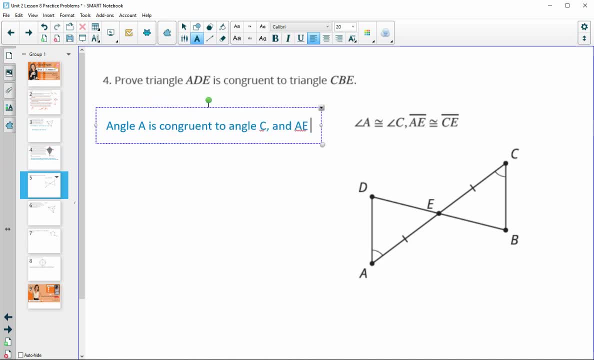 angle C B E. So we know that angle A is congruent to angle C B E. So they give us And A E segment. A E is congruent to segment C E because it was given to us. 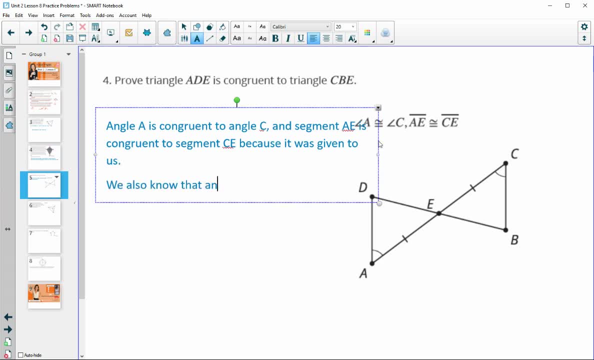 We also know that angle D, E, A. So this angle here is congruent. so DEA is congruent to BEC because they're vertical angles. therefore triangle ADE is congruent to triangle CBE by angle side angle triangle congruence. 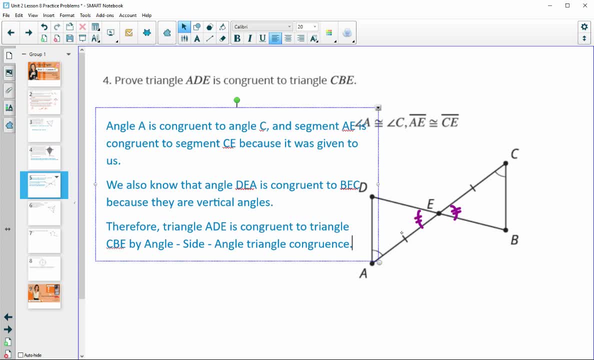 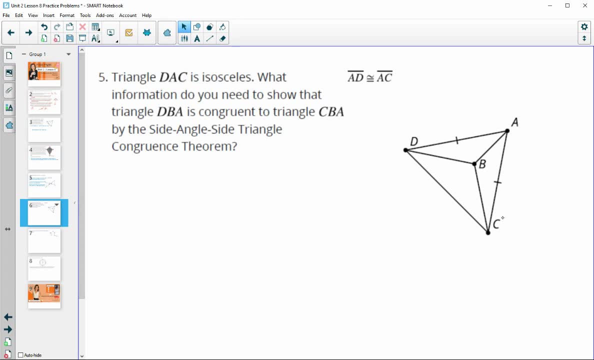 since we see that we have two angles with the side in between. number five, triangle DAC is isosceles. what information do you need to show that triangle DBA is congruent to CBA? so we want to prove that these two triangles here are congruent to each other with side angle side theorem. okay, so we want to get side angle side. so 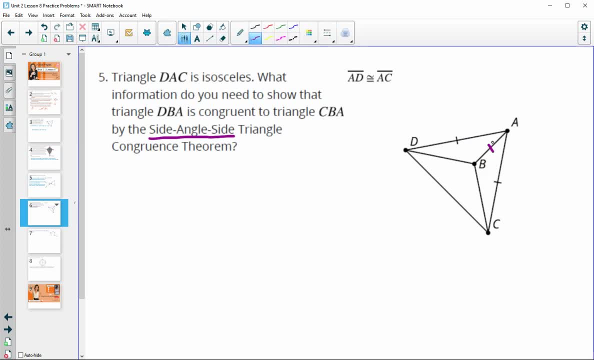 let's remember, if we're trying to prove those two congruent, AB is in both of them. so we would know that side angle, side theorem, is congruent. so the other thing that we need to know is: these two angles are congruent. so you could just straight up say that. so you could say: I need to know. 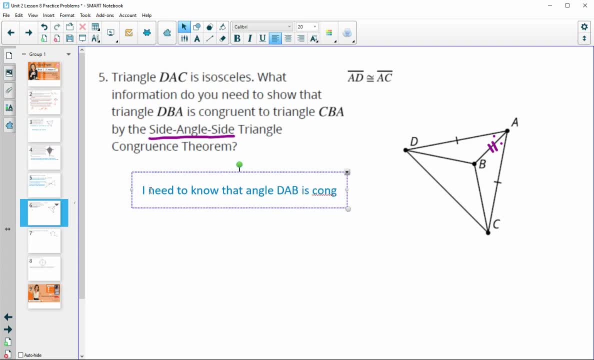 that angle DAB is congruent to angle CAB. so you could say that, or, if you wanted, you could just say so, or we could say that AB is the angle bisector, angle DAC. So either way, it gets you to the same spot, but they told you as the angle bisector. 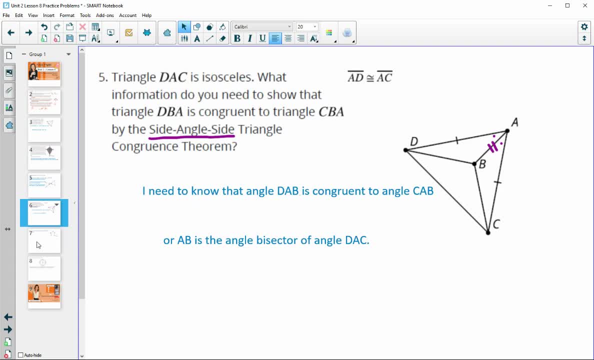 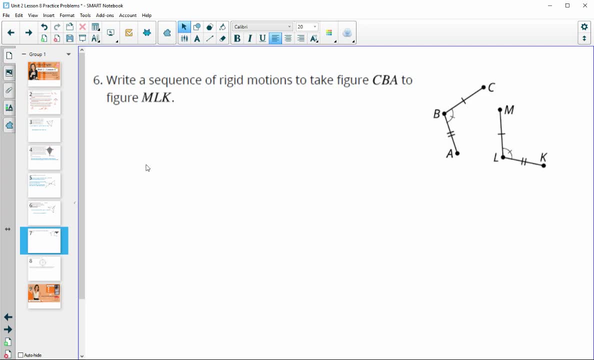 you'd know these two angles are congruent. or you could just say: I need to know those two angles are congruent because that's the meat of it. Write a sequence of rigid motions that would take CBA on to figure MLK. So we need to get them touching. So we're going to need to. 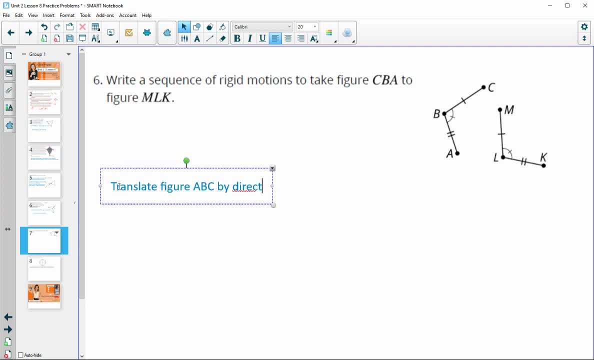 translate figure ABC by directed line segment and you can pick what you want. I'm going to get A to land on K, so AK, Then rotate the image of ABC until the image of B coincides with L. So I moved A on to K and then I rotated it until B landed on L. 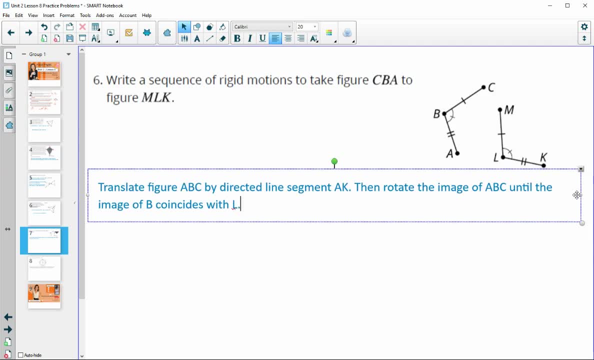 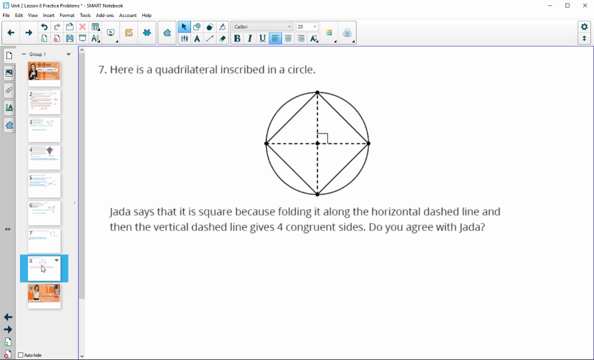 and then, And that'll get you to have the whole thing on top of you- That'll get ABC to land on KLM. All right, then we have this quadrilateral inscribed in a circle. Jada says that it is a square, because folding it along the horizontal dashed line and the vertical dashed line gives us four congruent sides. 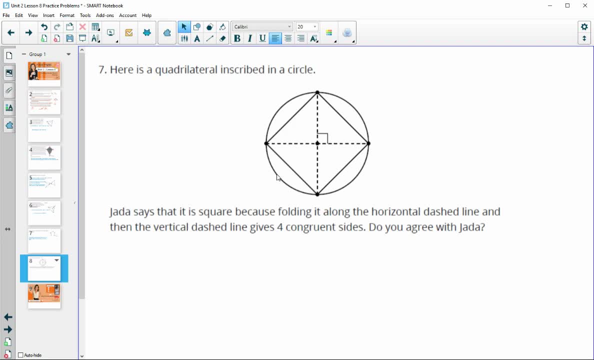 Do you agree with Jada? So it is a square, but she's kind of lacking a little bit in the explanation because she only got us four congruent sides. We also have to talk about these angles being right angles. So her conclusion is correct, but she didn't justify the quadrilaterals angles.